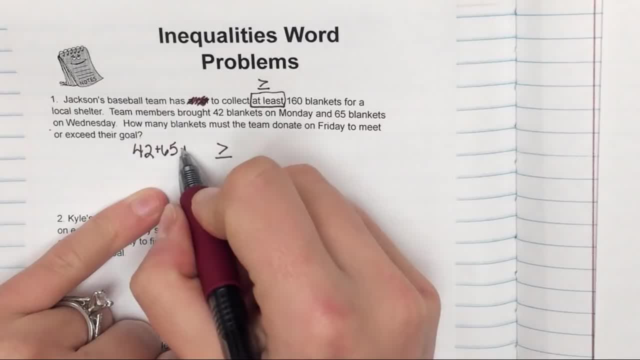 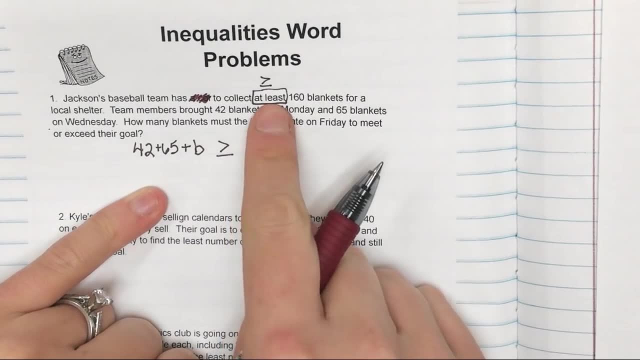 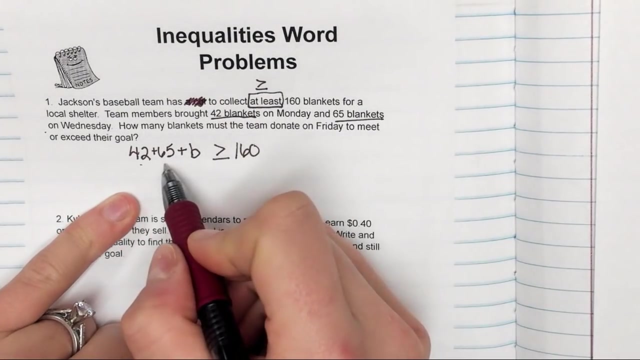 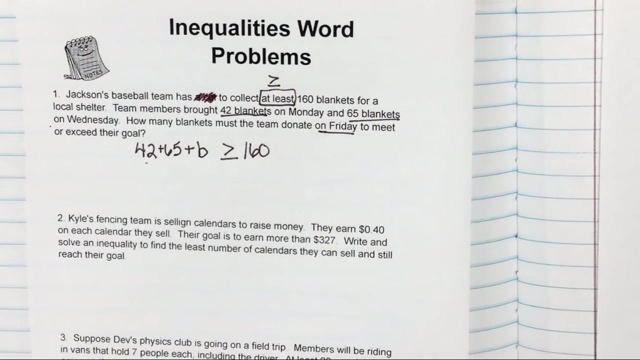 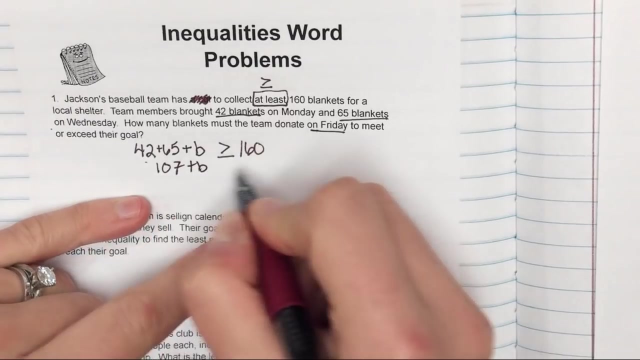 Plus, the team brings in some number of blankets, We're going to call that B on Friday. We want this to be greater than or equal to, So at least 160.. So again, 42 blankets on Monday, 65 blankets on Wednesday, And we want to know how many blankets on Friday, And that's where our variable is going to be. So to solve this inequality, I have 42 plus 65. And that gives me 107. plus B is greater than or equal to 160. 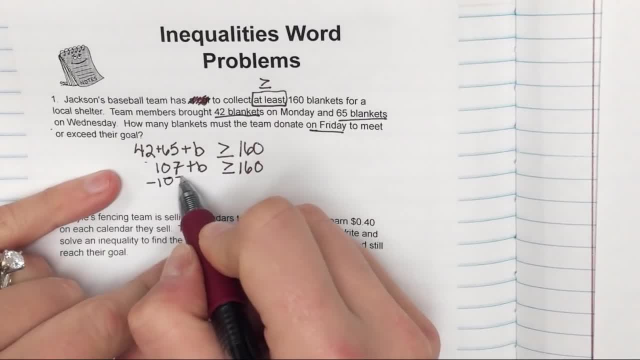 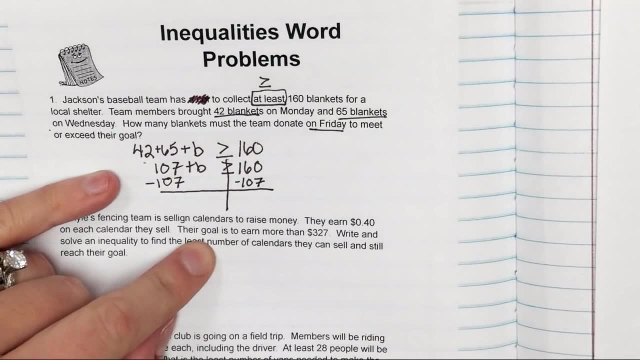 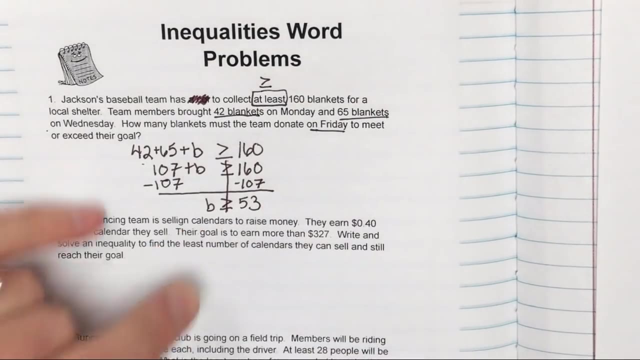 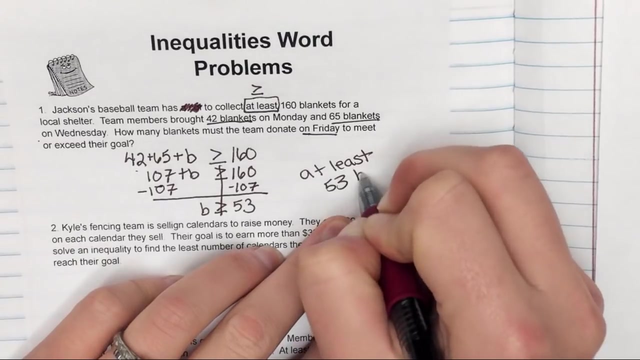 I'm going to use the subtraction property of inequality and I'm going to subtract 107 from both sides. So 160 minus 107 gives me 53. So I have B is greater than or equal to 53. So the answer to this word problem would be at least 53 blankets. 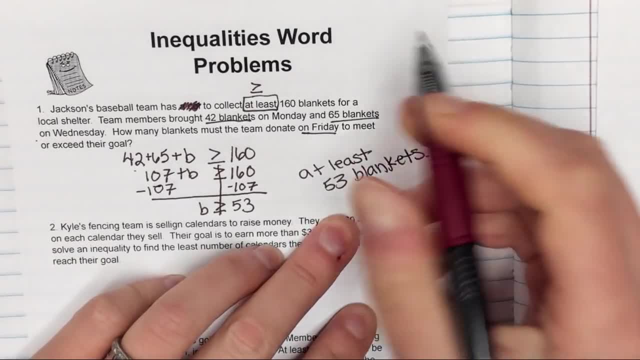 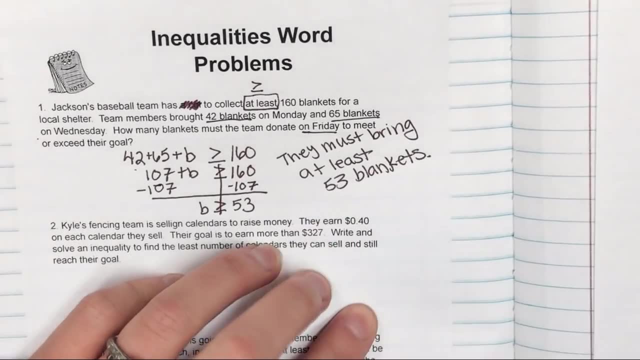 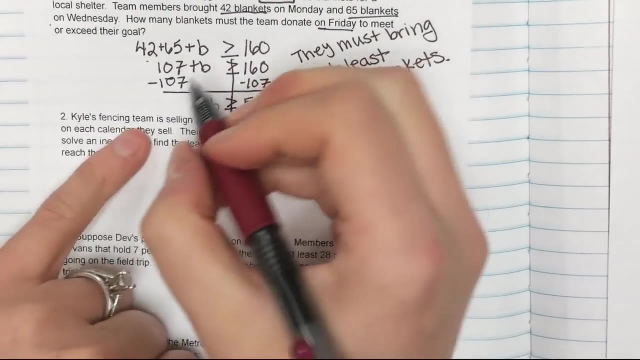 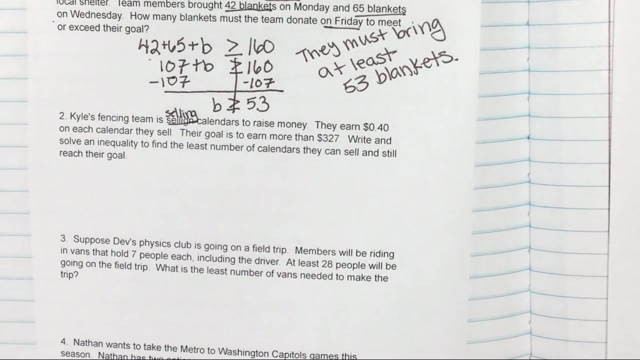 Let's answer that in a complete sentence. We must bring at least 53 blankets Alright. number two, Kyle's fencing team is selling. Wow, I'm all kinds of typos today Selling calendars to raise money. They earn 40 cents on each calendar they sell. 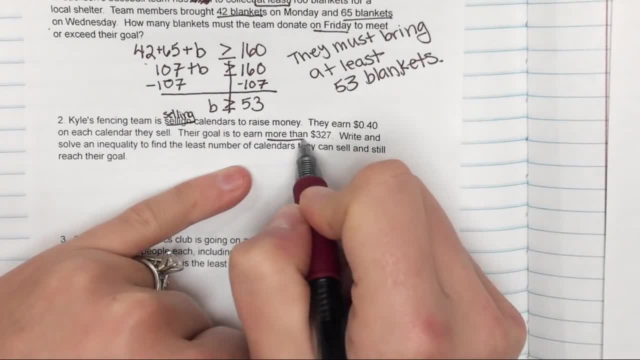 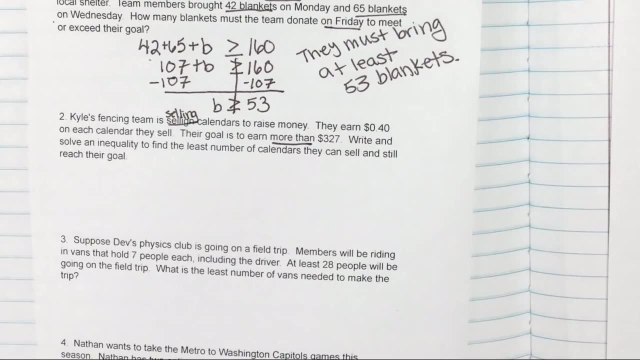 Their goal is to earn more than there's your inequality word: more than $327.. Write and solve an inequality to find the least number of calendars They can sell and still reach their goal. More than is a greater than word. You want to earn more than. 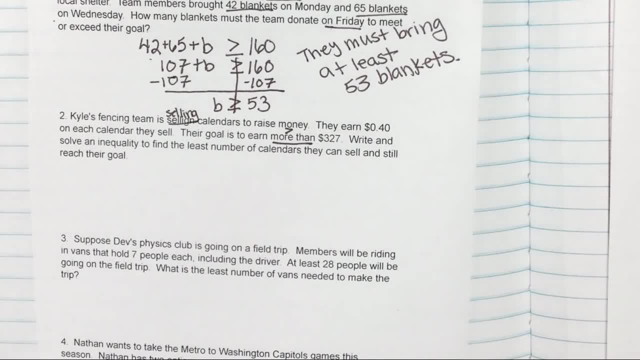 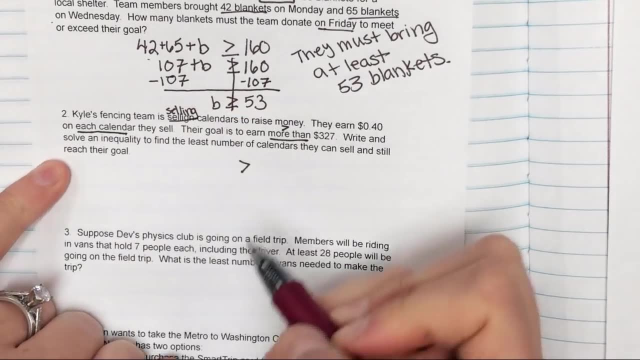 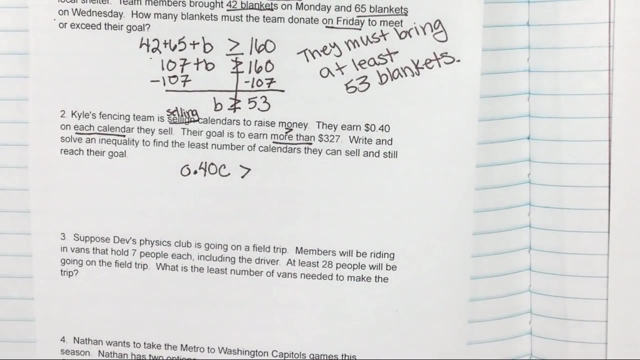 Not, at least. you want to have more than $327. So we know we're going to have greater than We earn. 40 cents on each calendar. So 40 cents for each calendar. Each is either a multiply or divide word, depending on the context of the problem. 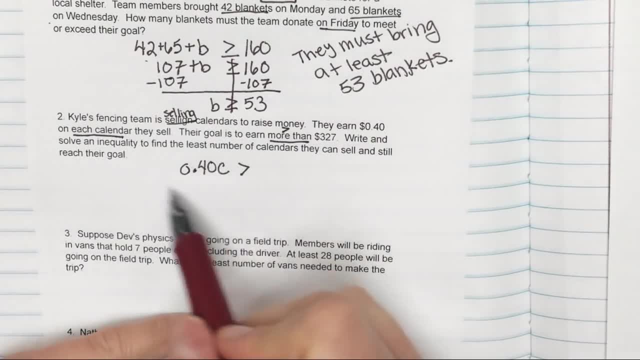 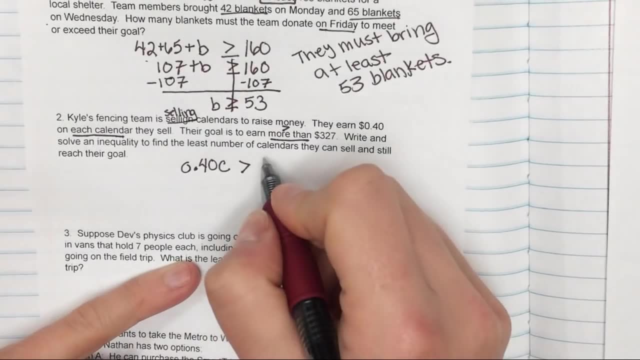 In this case, because we're going to be selling, we're going to have $327.. And because we're selling many, many, many calendars, it's going to be a multiplication word. So 40 cents times the number of calendars sold has got to be greater than $327.. 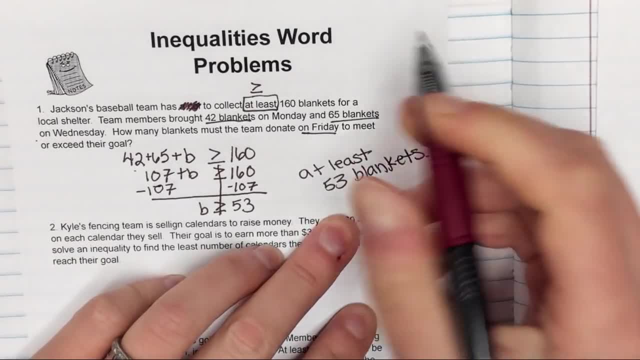 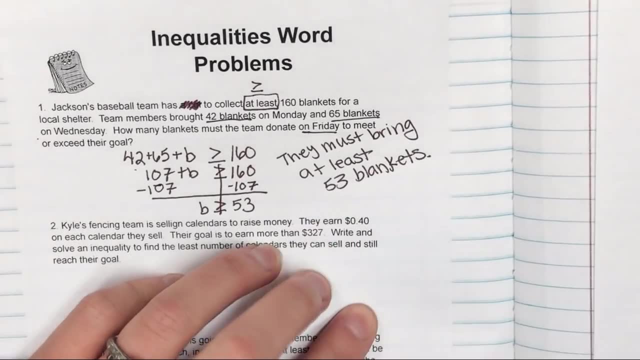 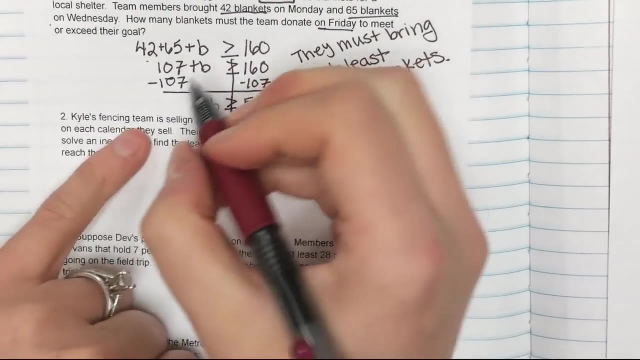 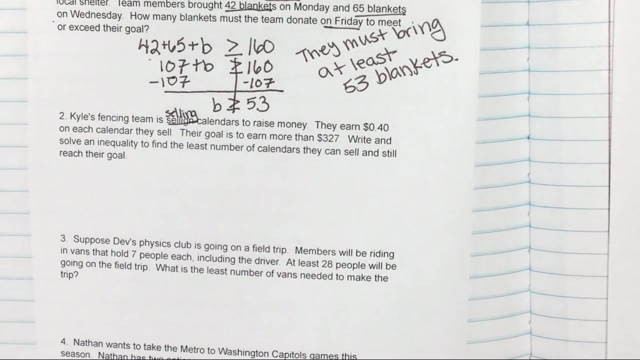 Let's answer that in a complete sentence. We must bring at least 53 blankets Alright. number two, Kyle's fencing team is selling. Wow, I'm all kinds of typos today Selling calendars to raise money. They earn 40 cents on each calendar they sell. 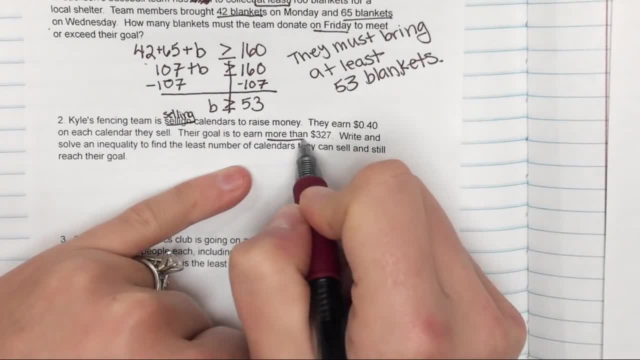 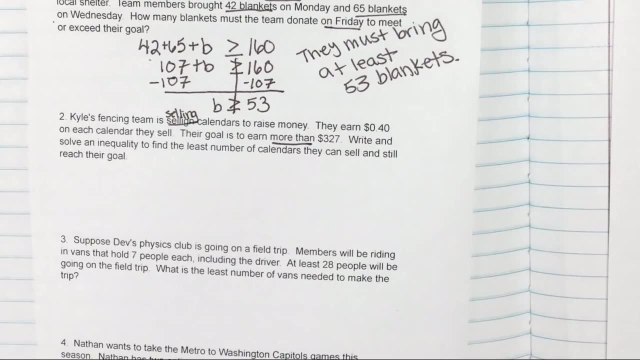 Their goal is to earn more than there's your inequality word: more than $327.. Write and solve an inequality to find the least number of calendars They can sell and still reach their goal. More than is a greater than word. You want to earn more than. 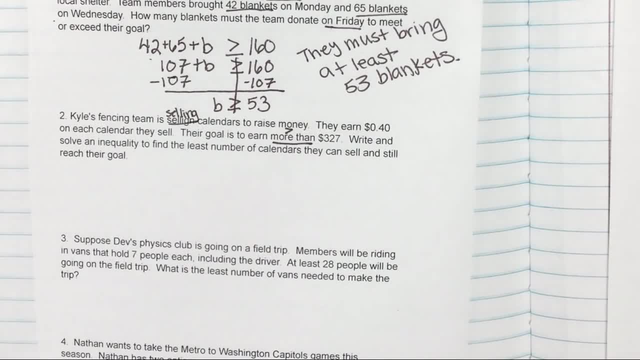 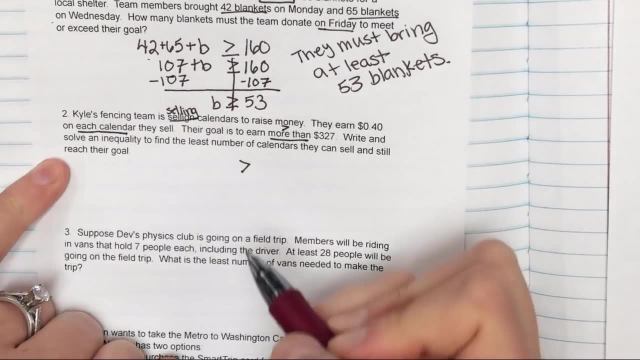 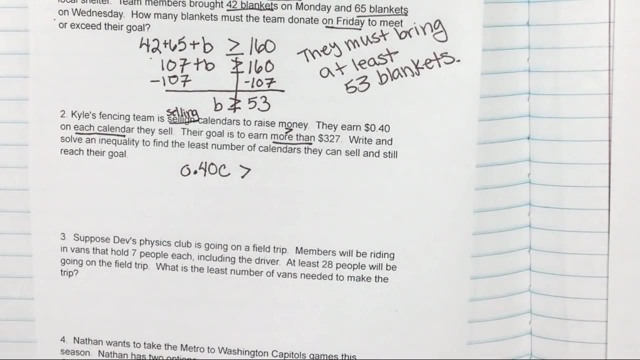 Not, at least. you want to have more than $327. So we know we're going to have greater than We earn. 40 cents on each calendar. So 40 cents for each calendar. Each is either a multiply or divide word, depending on the context of the problem. 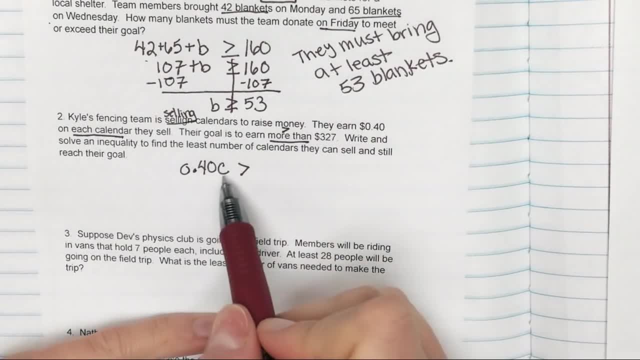 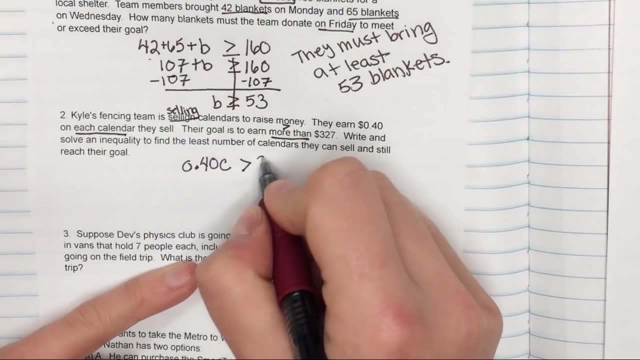 In this case, because we're doing the math, we're going to have a multiply or divide word. we're selling many, many, many calendars. it's going to be a multiplication word. So 40 cents times the number of calendars sold has got to be greater than $327.. So, in order, 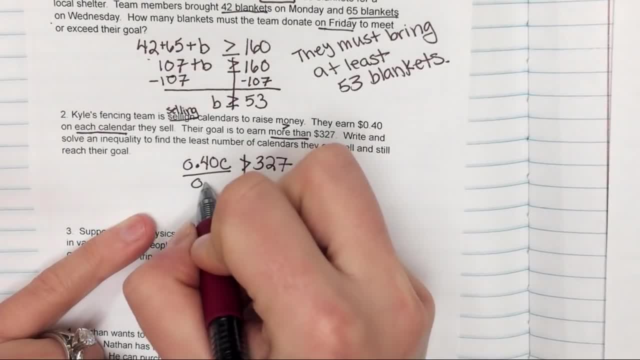 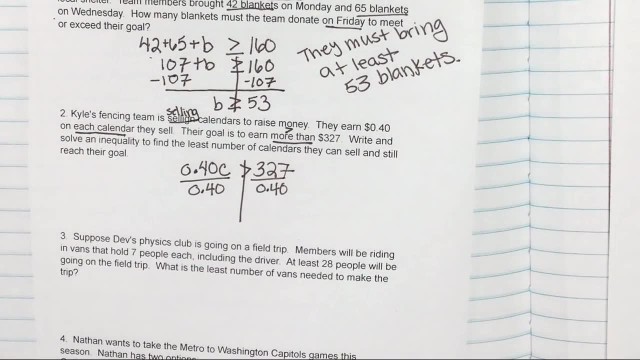 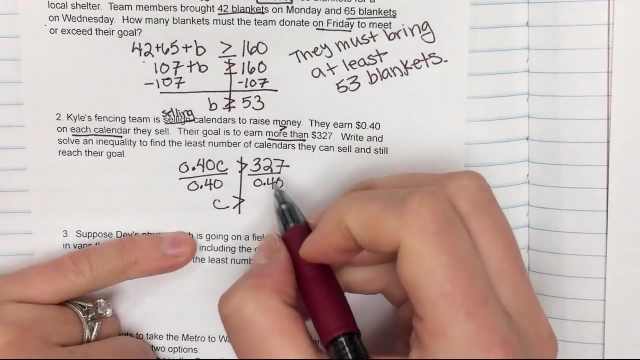 to solve this I'm going to use the division property of inequality and I'm going to divide by 0.40.. So 327 divided by 0.40 gives me C is greater than 817.5.. Now I need to think. 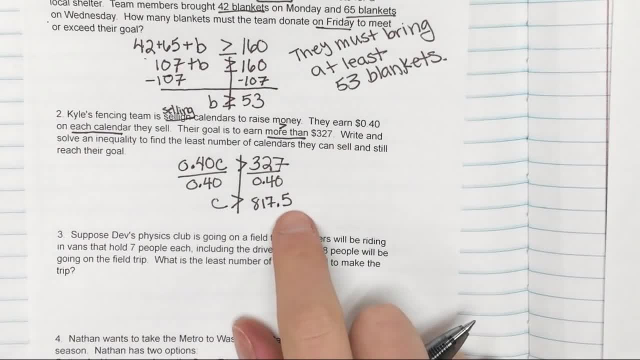 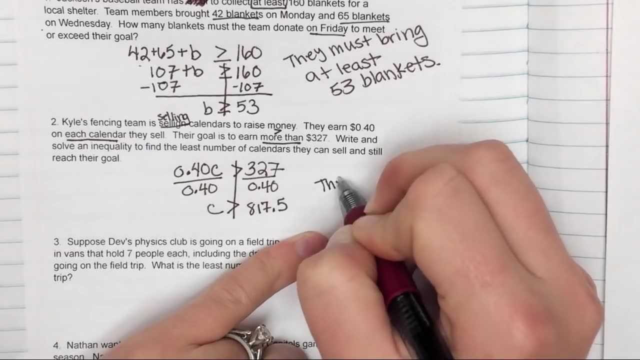 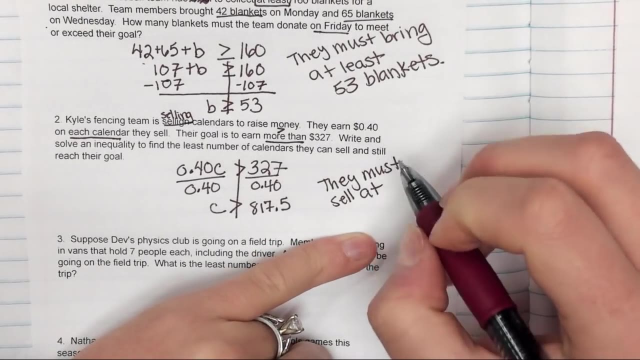 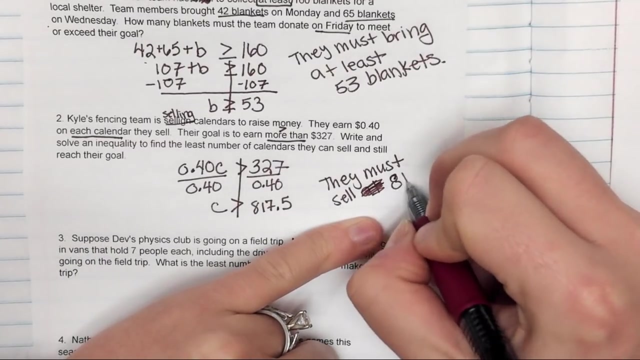 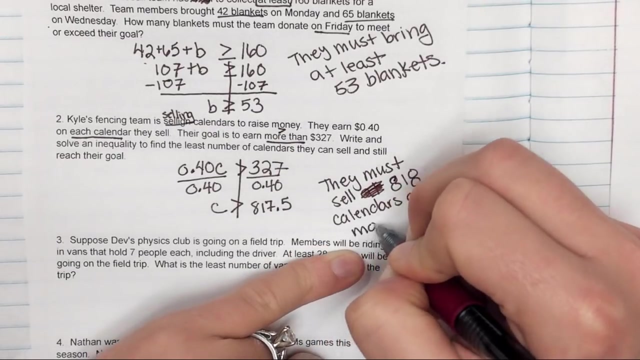 about this. Is it possible to sell half a calendar? No, So I'm going to need to round this up to 318.. So they have must sell at. they must sell 3, 800,- sorry, 818 calendars or more to meet their goal. 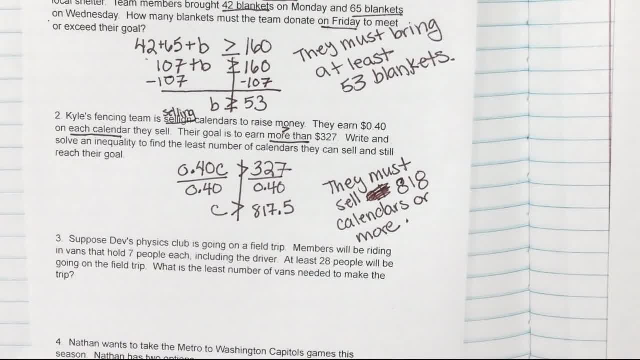 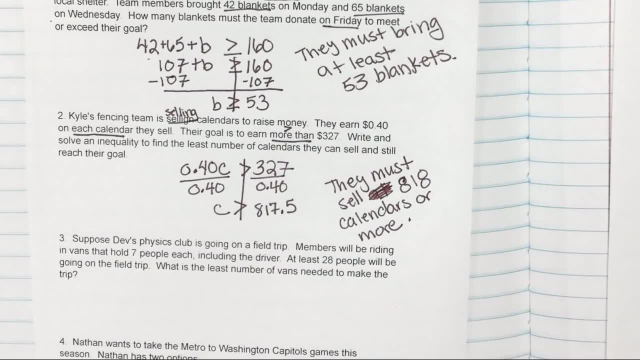 They must sell 818 calendars or more. Again, you can't sell part of a calendar and somebody would be very unhappy if they got a calendar that only went January through June and you're missing July through December. So we're not selling. 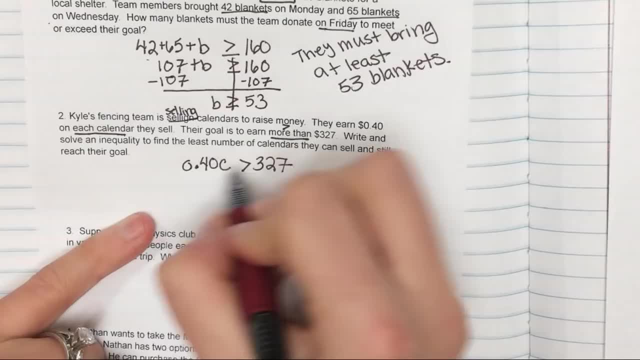 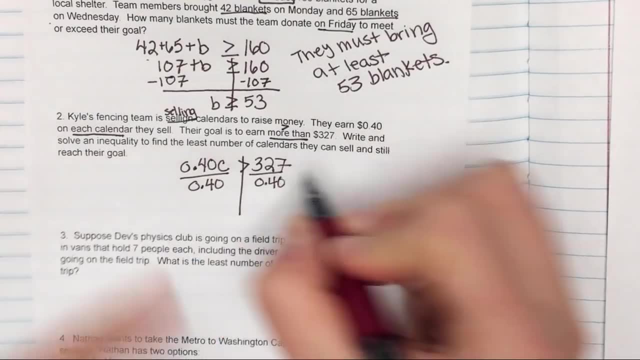 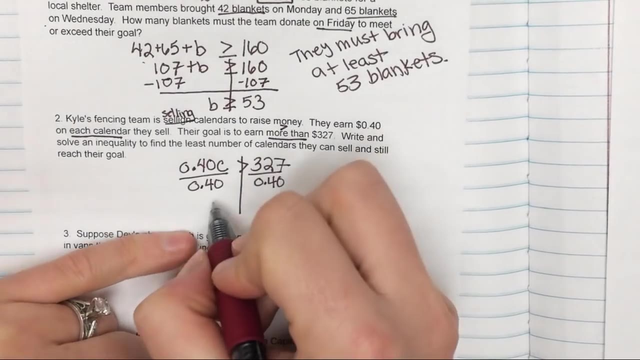 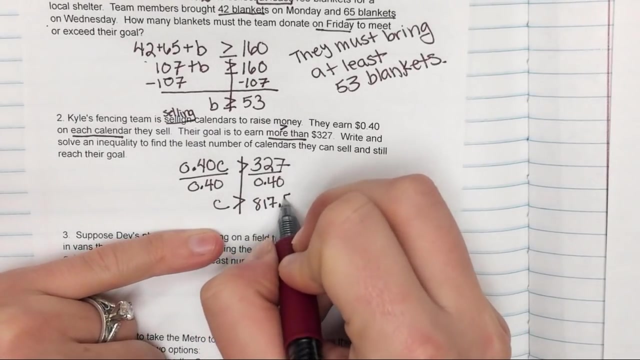 So, in order to solve this, I'm going to use the division property of inequality and I'm going to divide by 0.40.. So 327 divided by 0.40 gives me C is greater than $327.. C is greater than $817.5. 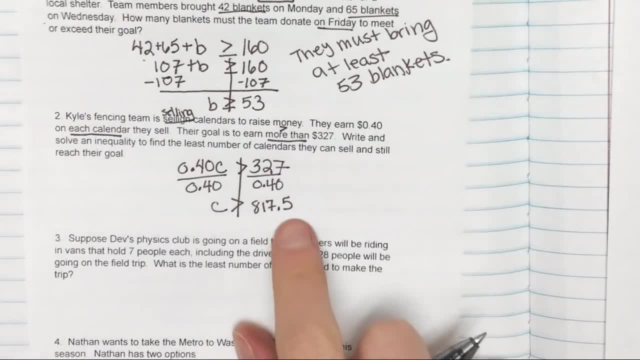 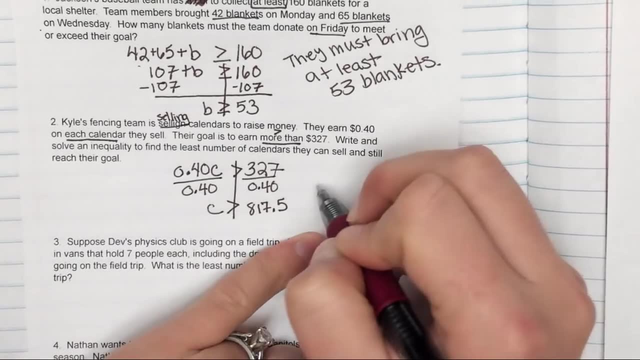 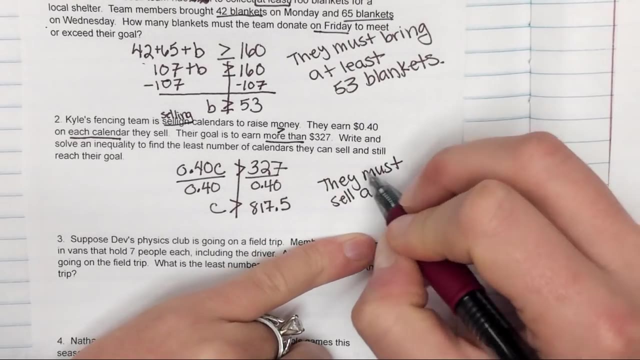 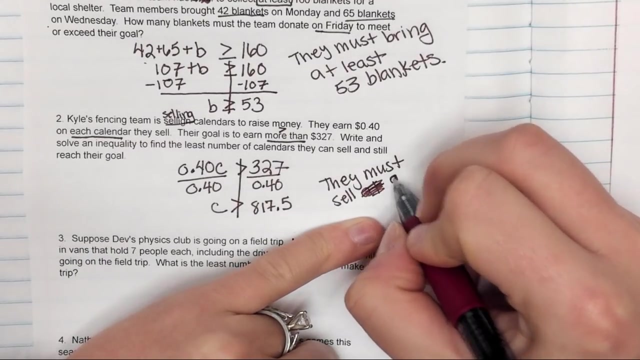 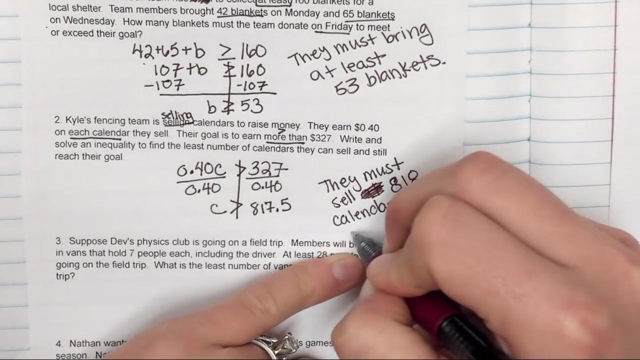 Now I need to think about this: Is it possible to sell half a calendar? No, So I'm going to need to round this up to $318.. So they must sell at. They must sell $318.. Sorry, $818 calendars or more to meet their goal. 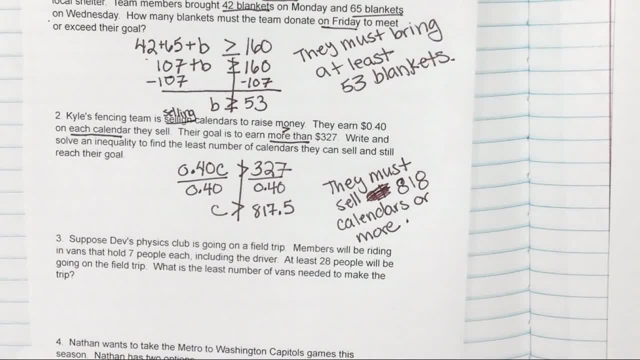 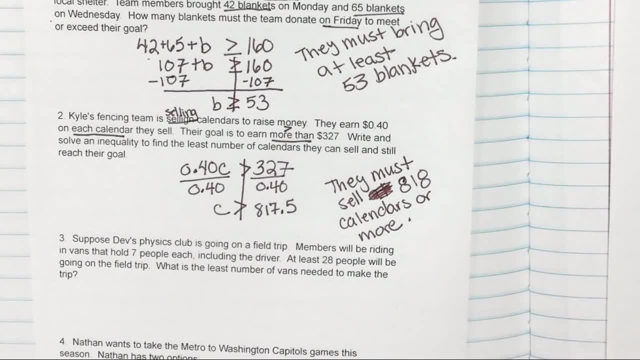 They must sell 818 calendars or more. Again, you can't sell part of a calendar. Somebody would be very unhappy if they got a calendar that only went January through June and you're missing July through December. So we're not selling half a calendar rounding up to the nearest whole number. 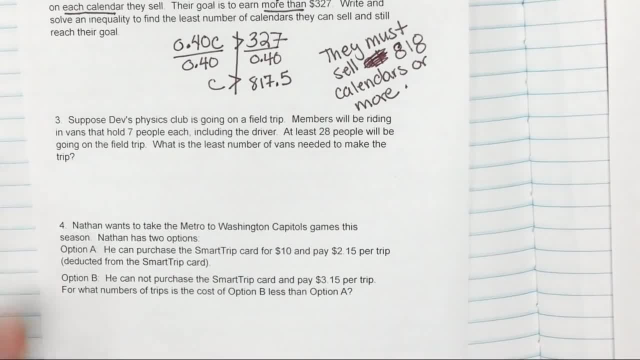 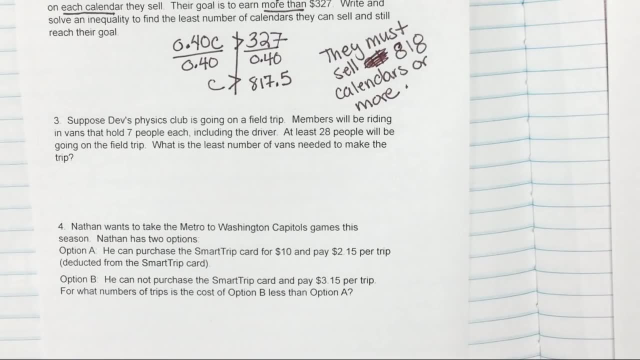 All right. next question three: Suppose Dev's Physics Club is going on a field trip. Members will be riding in vans that hold seven people each, including the driver. At least 28 people will be going on the trip. What is the least number of vans needed to make the trip? 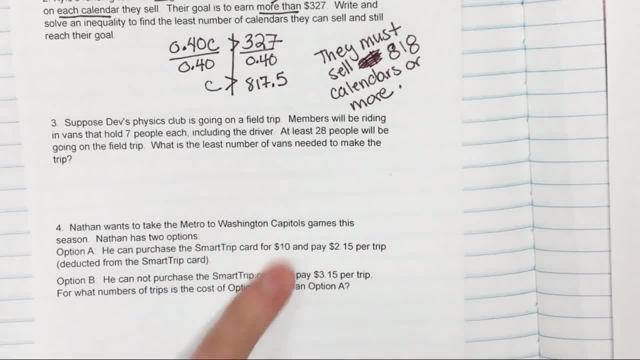 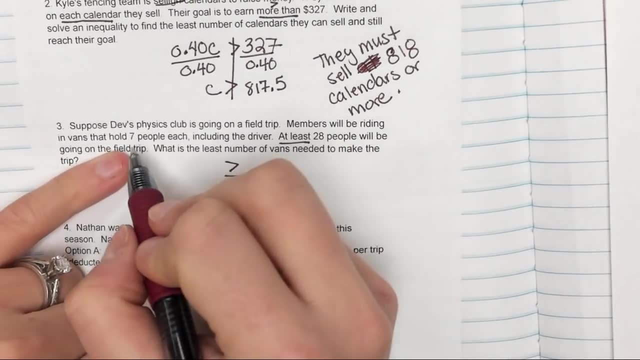 Okay, so at least 28 people. Again, that's a greater than or equal to word. So we know we're going to need greater than or equal to. These vans hold seven people each, so we're going to have 7 times V. 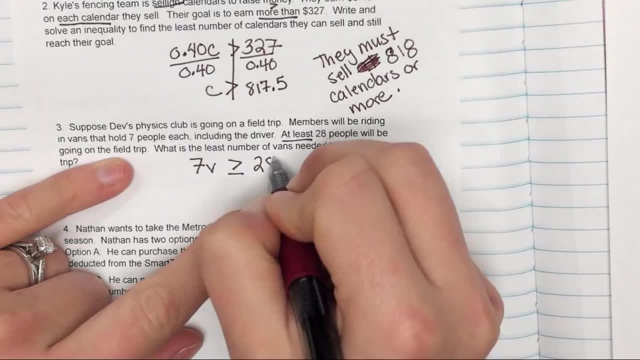 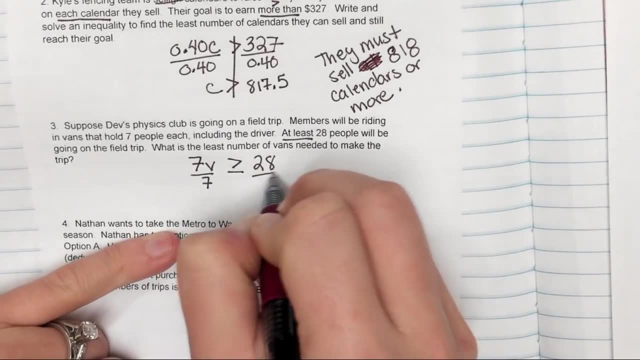 And we know that at least 28 people are going And we're looking for the minimum number of vans. So now I'm going to use the division property of inequality. I'm going to divide both sides by 7. And I have V is greater than or equal to 4.. 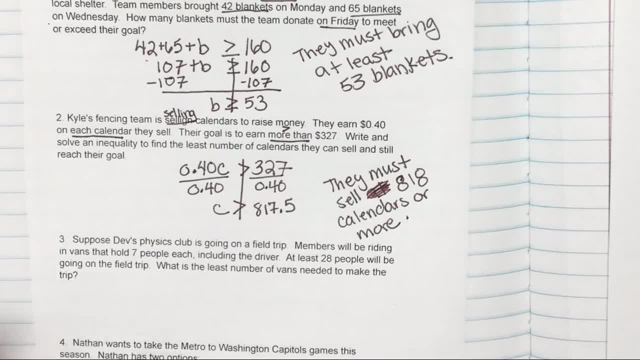 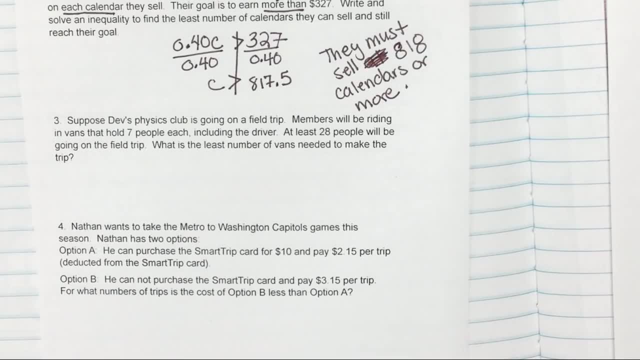 half a calendar rounding up to the nearest whole number. Alright, next question three: Suppose Dev's Physics Club is going on a field trip. Members will be riding in vans that hold seven people each. including the driver, At least 28 people. 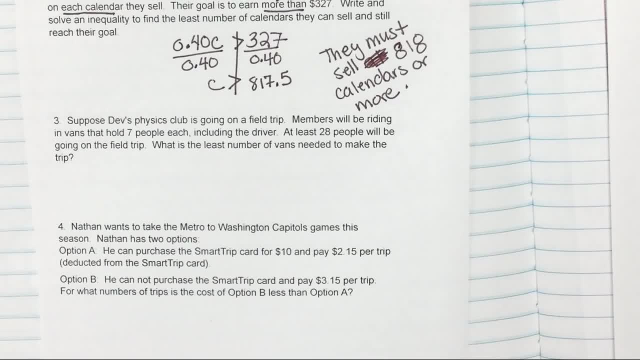 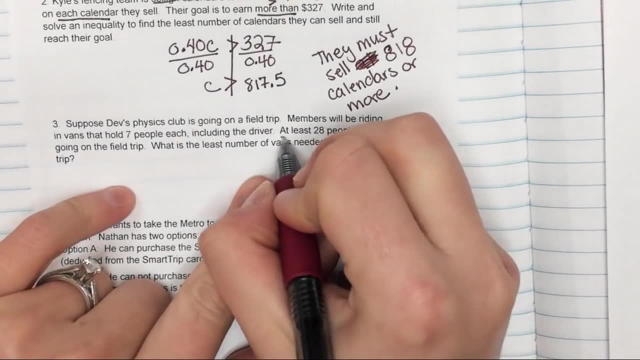 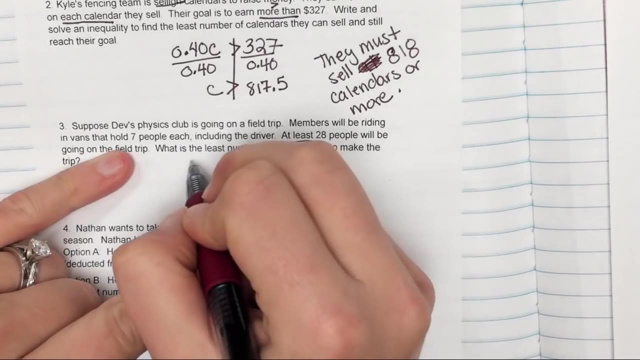 will be going on the trip. What is the least number of vans needed to make the trip? Okay, So at least 28 people. Again, that's a greater than or equal to word. So we know we're going to need greater than or equal to. These vans hold seven people each, so we're going to 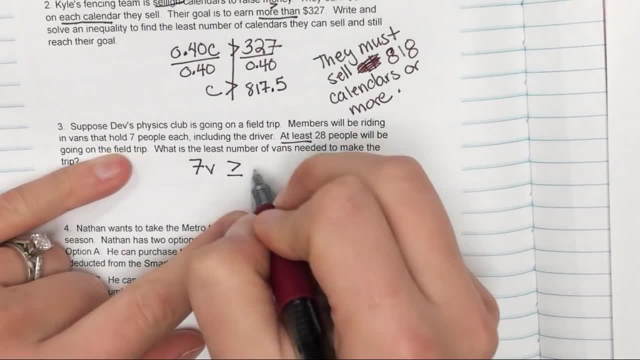 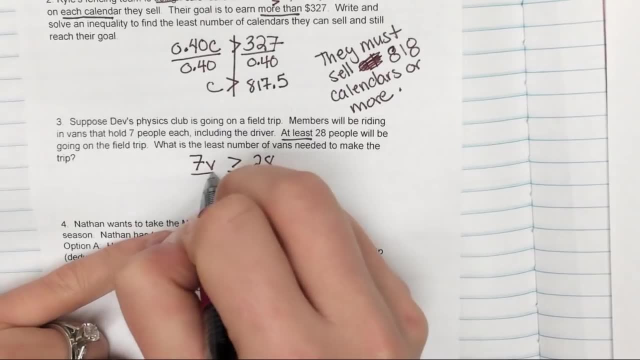 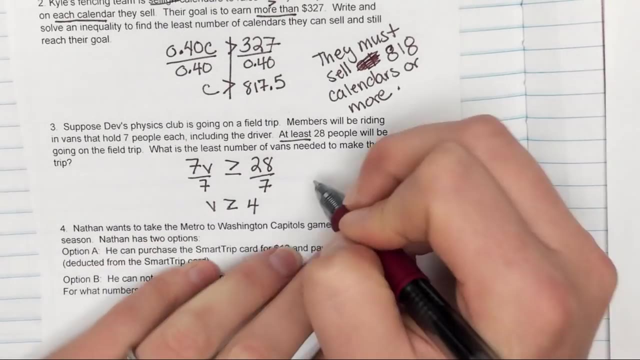 have seven times v and we know that at least 28 people are going and we're looking for the minimum number of vans. So now I'm going to use the division property of inequality. I'm going to divide both sides by seven and I have v is greater than or equal to four. 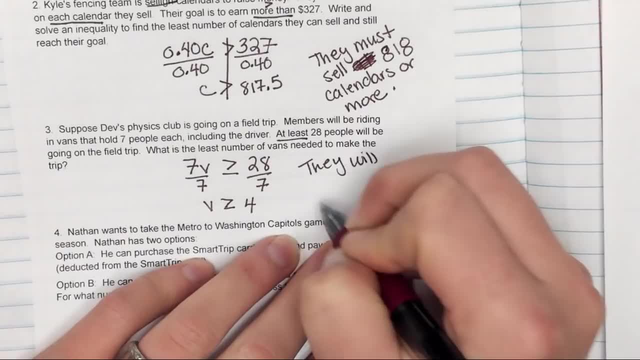 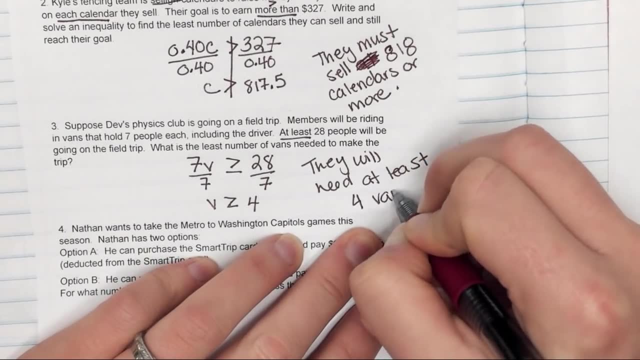 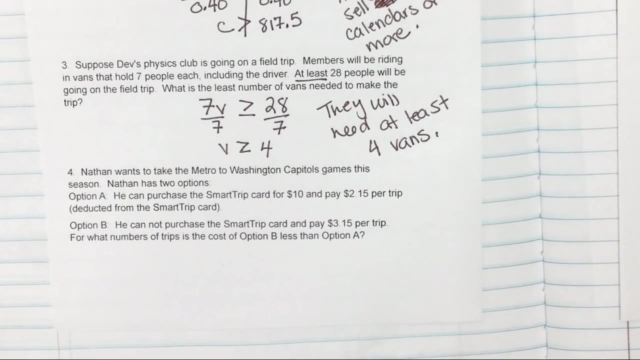 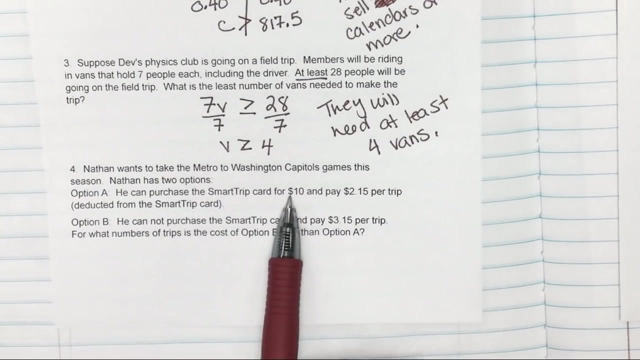 So they will need at least four vans. Alright, number four: Nathan wants to take the Metro to Washington to the Washington Capitals game this season. Nathan has two options. Option A, he can purchase the Smart Trip card for $10 and pay $2.15 per trip. Or option B, he could not purchase the Smart. 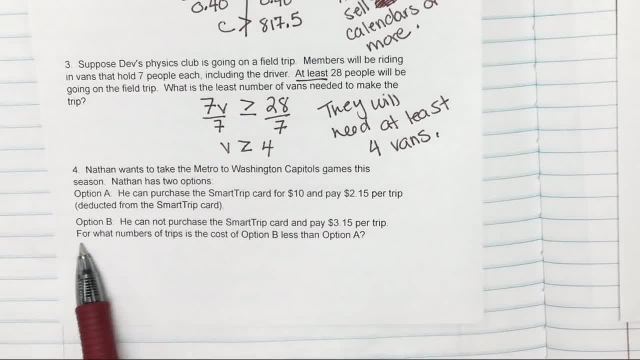 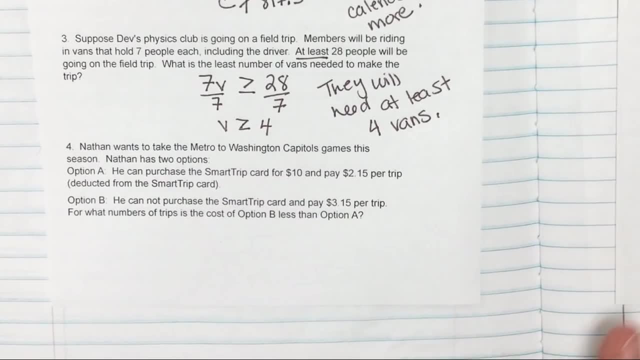 Trip card and pay $3.15 per trip. For which number of trips is the cost of option B? the option A less than the cost of option A? Okay, so let's talk about cost of option B, since it's less than we're going to use less. 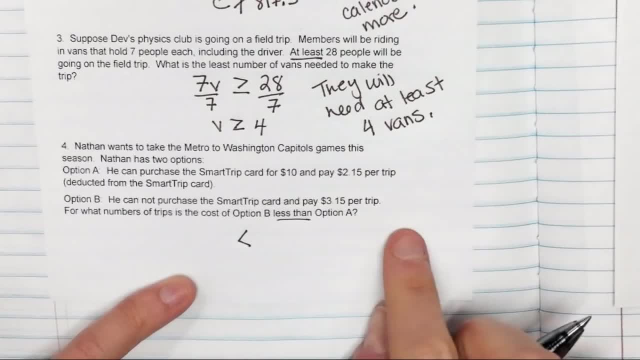 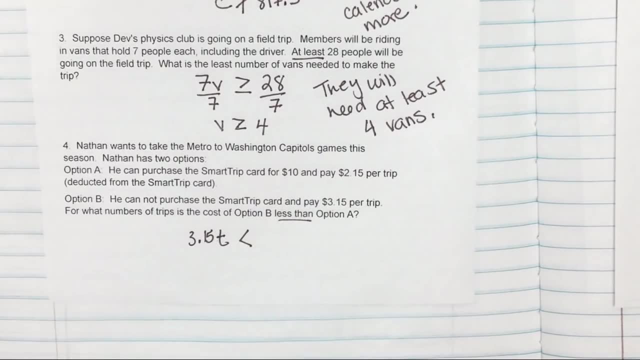 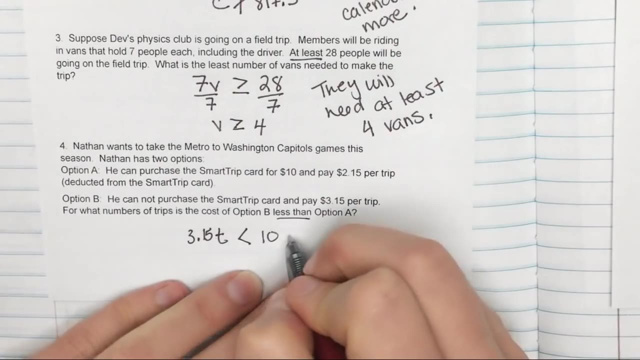 than- and we're starting with option B- is less than option A. So option B is $3.15 times the number of trips and I'm going to use T for trips. Option A is a $10 flat fee to buy the card, and then we're adding to that cost $2.00. 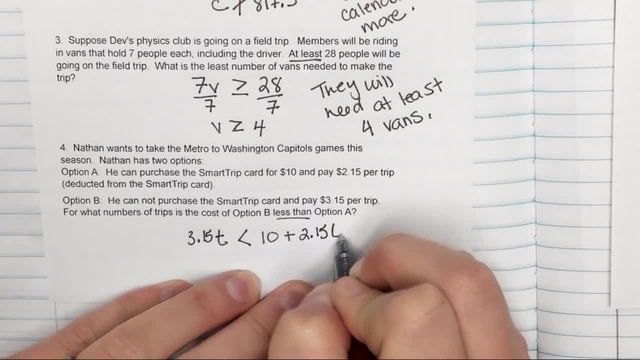 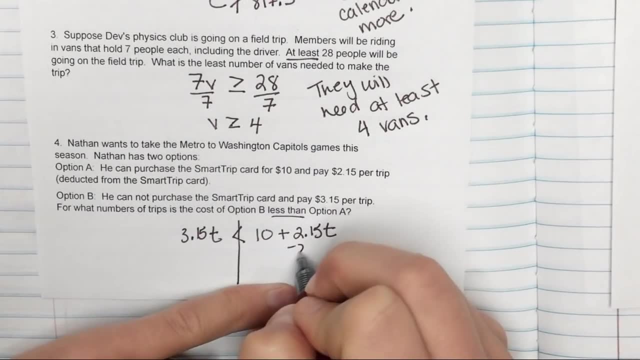 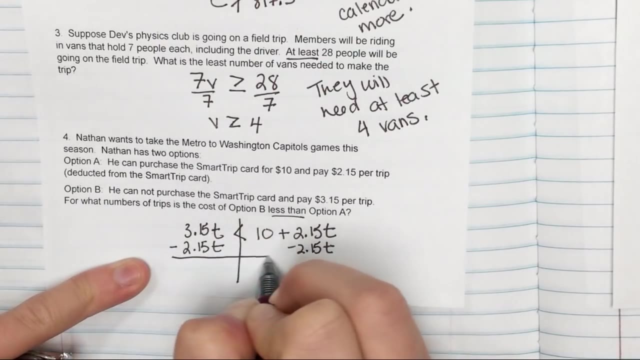 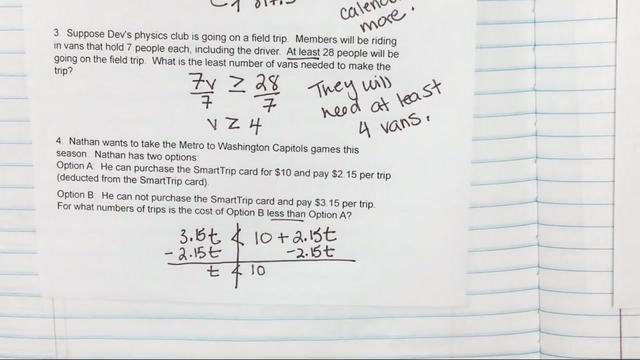 per drop off and 15 cents for each trip that he takes. So I'm going to solve this inequality for T by subtracting two dollars and 15 cents times T from both sides. So this is going to leave me with just T is less than 10.. So option B is cheaper. if Nathan takes less than 10 trips. If Nathan takes less than 10 trips,